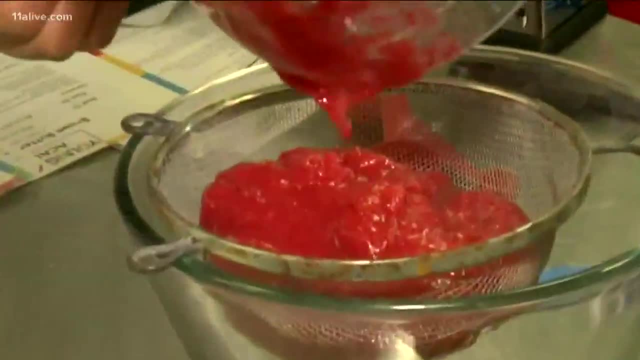 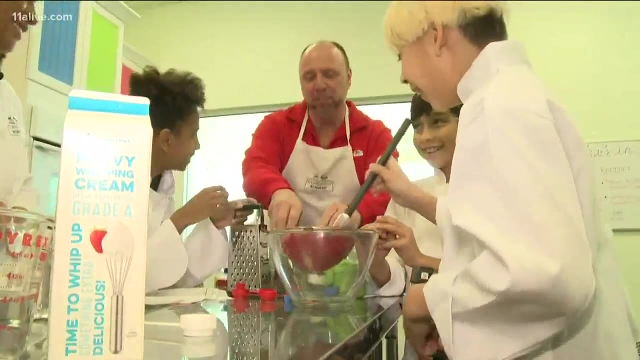 in there and use your knuckle man, you got to punch it rocky style. Get that spatula If you need someone to help you push it. salt and pepper, Push it, push it, push it real good. While the tart sets, it's on to the brown butter braised leeks. 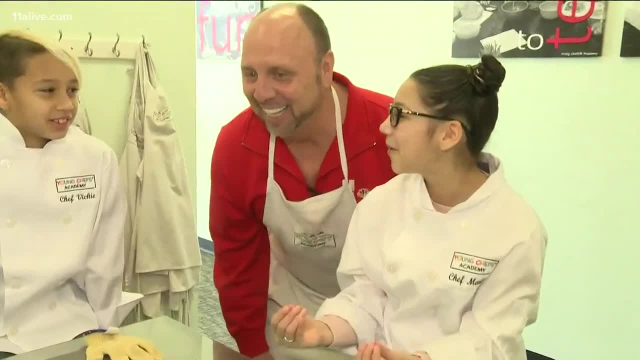 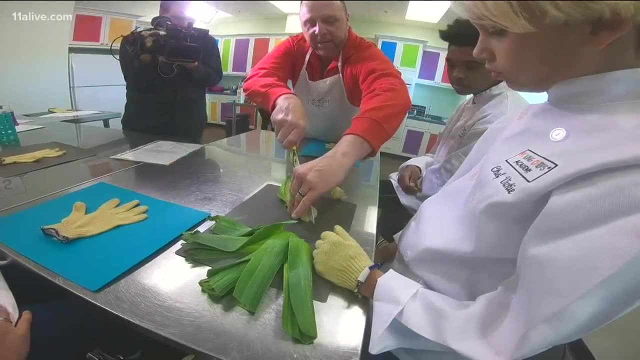 Say, when the boat had a hole, What? The boat is leaking. the boat is leaking. We're going to cut off the root and then slice it lengthwise. And you straddle it that way your fingers are away from it and you can just go right down the middle like 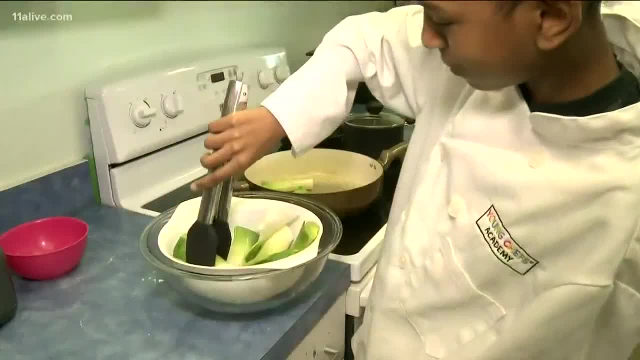 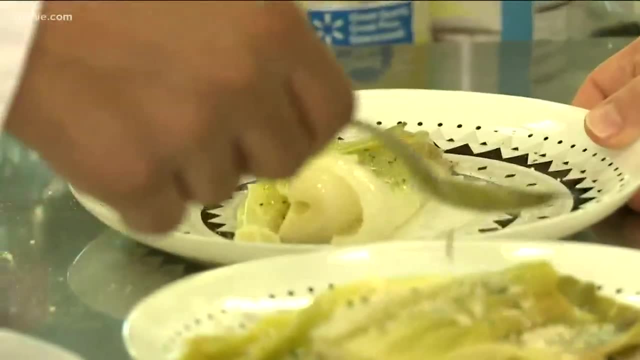 that and your fingers are away from where you're cutting. It kind of looks like a giant green onion. Are they somewhat in the same family? It is kind of in the same family. It has that same flavor also, kind of oniony garlicky. Yeah Yeah, really good flavor. 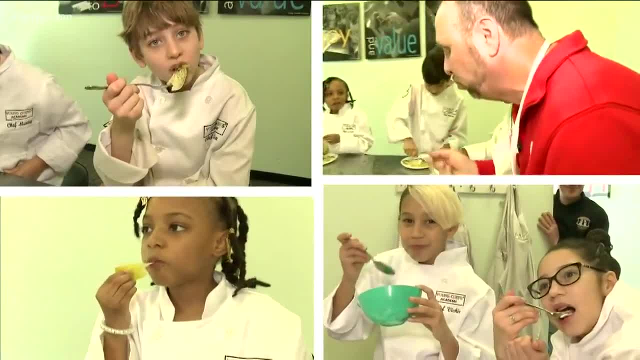 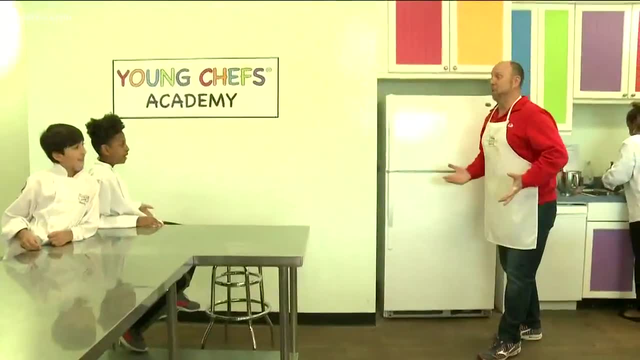 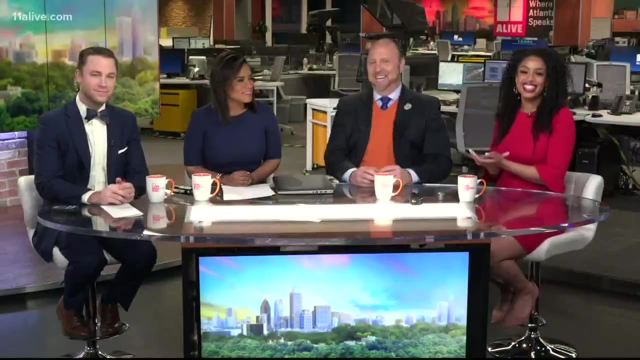 With the tart set and the leeks browned, it was time to taste our creations. Wow, Is it good. That's delicious, Thank you. Even though we're not supposed to run around after we eat, young chefs give it up What up. Yeah, It turned into quite a joke. session with the. 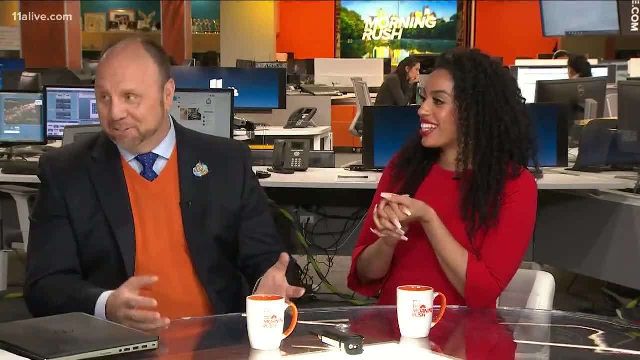 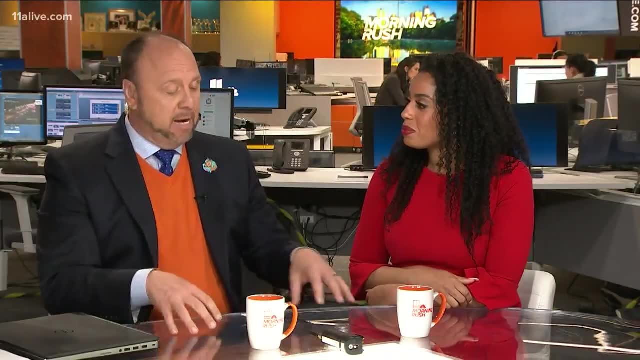 the little kids. once they realize, all we could do is tell funny jokes plus a lot of leak jokes- yeah, no, they were great. and I mean the Young Chefs Academy. there are several locations: Sandy Springs, there in Marietta, Midtown. they're actually getting ready to build another location, very popular- children as young 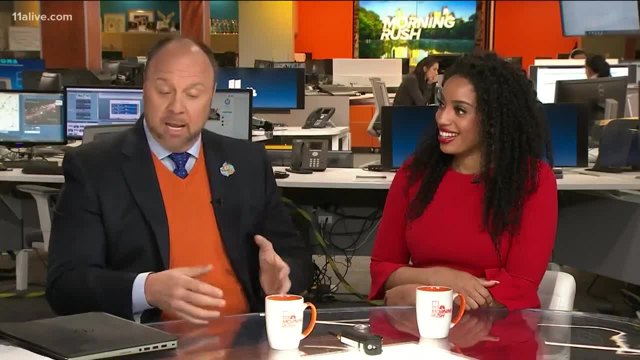 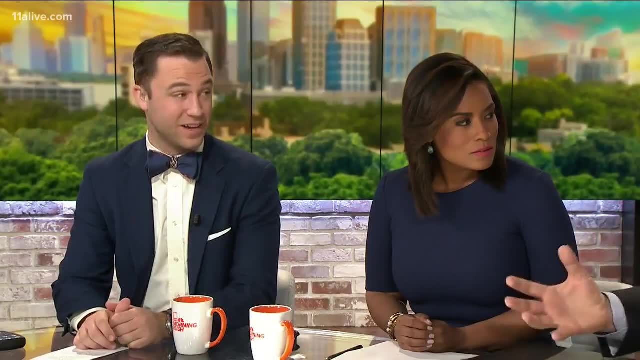 as four years old in the kitchen learning this and some of the parents were talking to me and they were saying: they wake up in the morning, they'll cook breakfast for the family. when they go shopping they'll purchase ingredients. I mean, it's amazing how these kids are just infused into their culinary world. 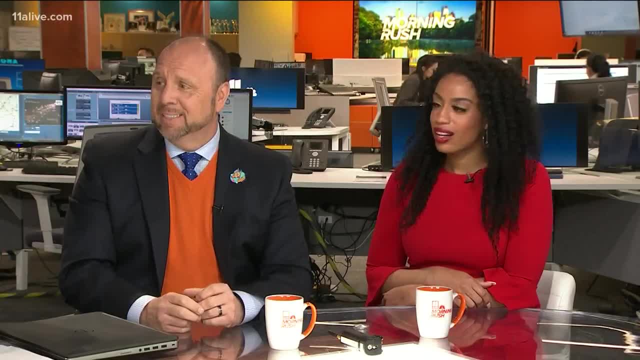 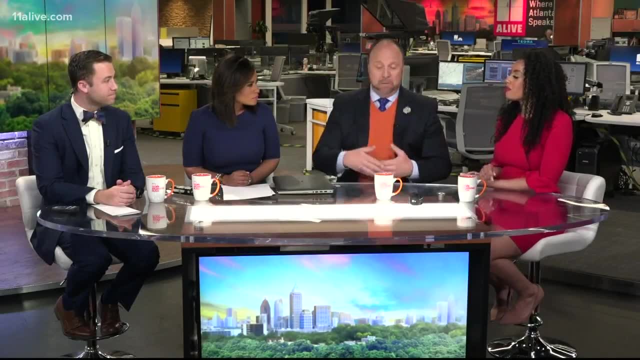 but the kids to work, right, yeah, big time. and you saw some teenagers there. you saw 16 year old. yeah, yeah, there was a, I think as old as 16 years old, wasn't it? so, yeah, I mean, if you're looking for something for the kids to do, either, a. 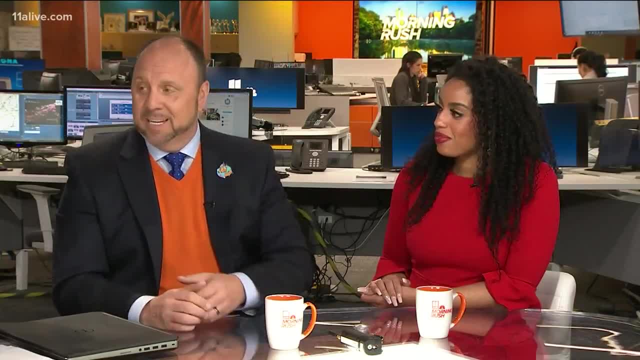 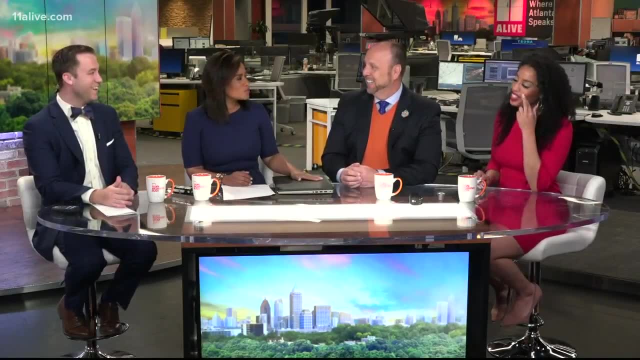 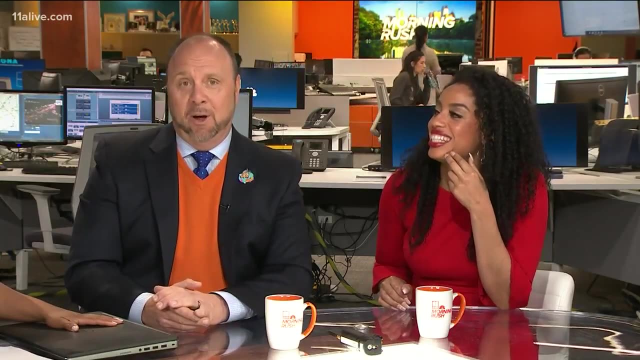 summertime thing, or almost out. yeah, I mean, it's a lot of fun. why not at the end of the summer? know that you have an in-house chef. you are so great with those kids. you could be like a teacher. we actually found my new demo. I'm gonna now start hitting the five to twelve year old audience here for the.